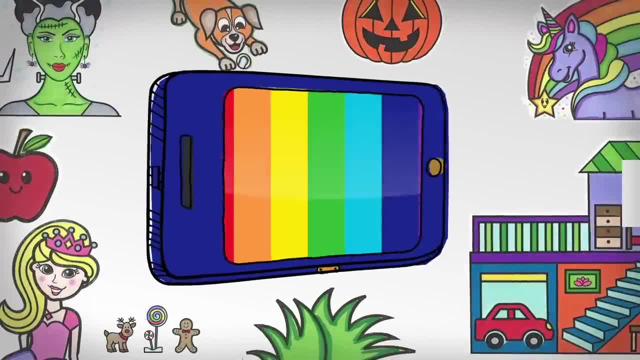 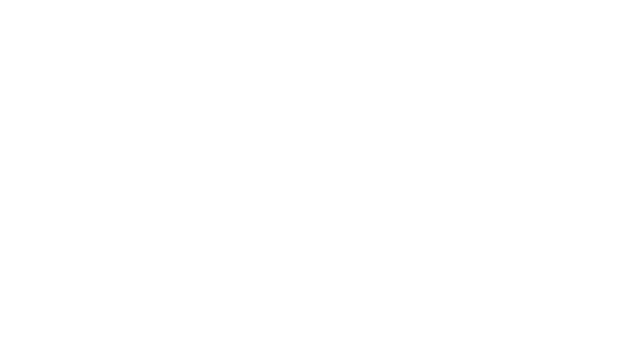 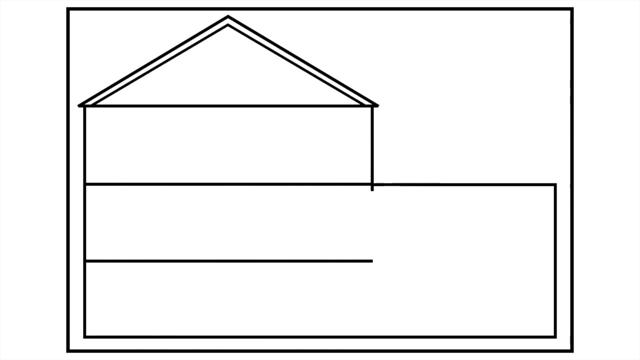 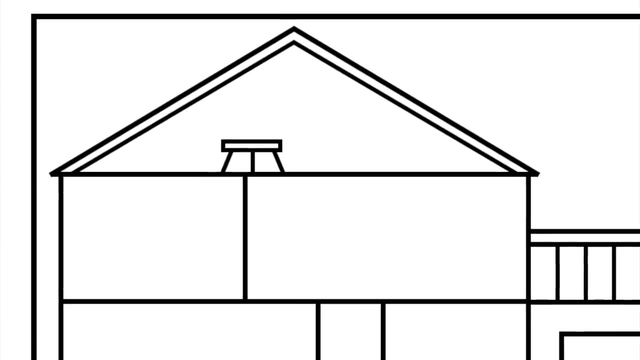 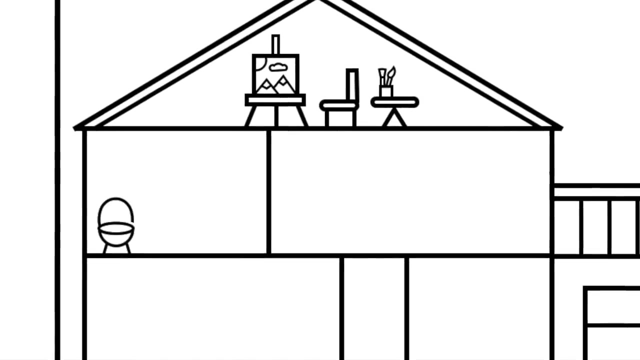 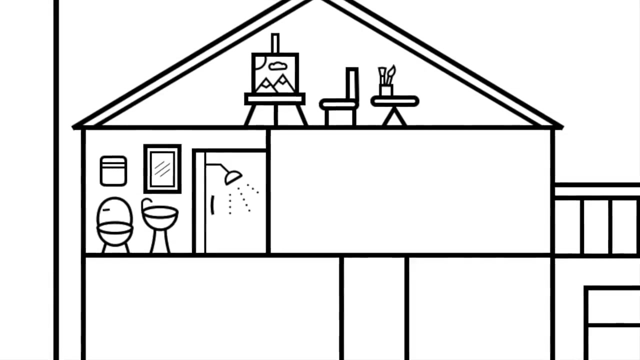 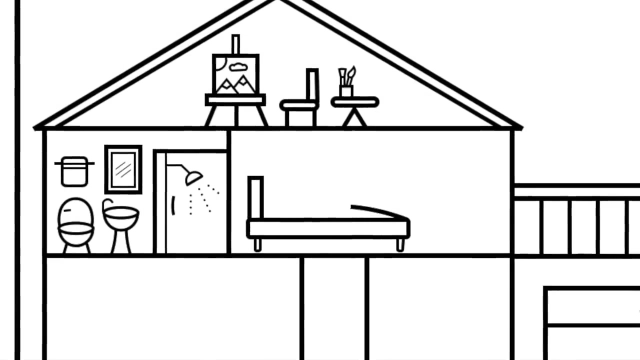 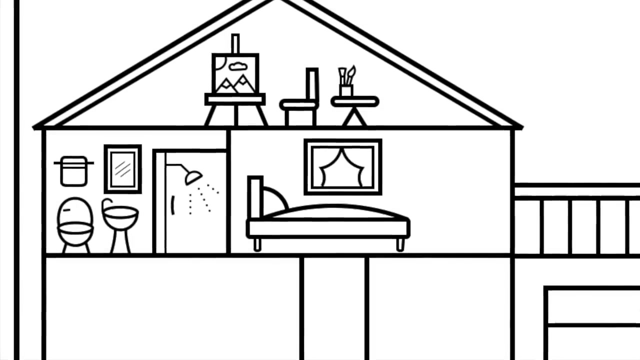 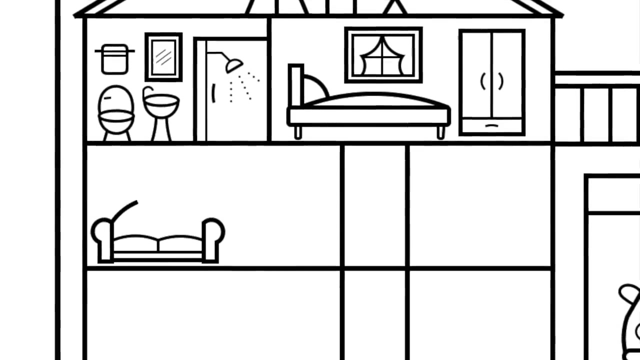 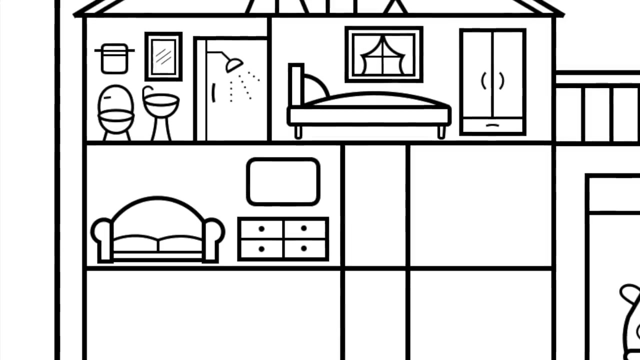 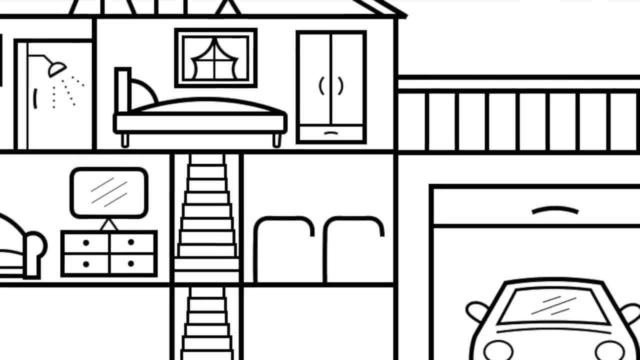 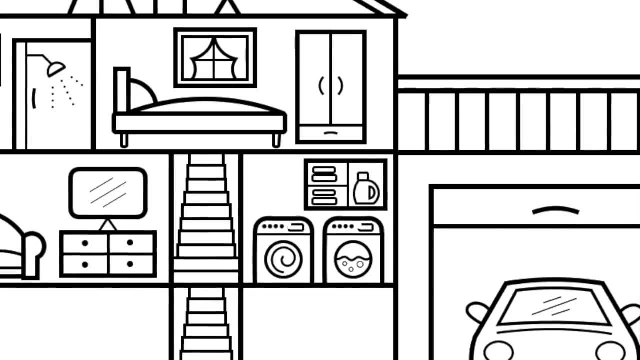 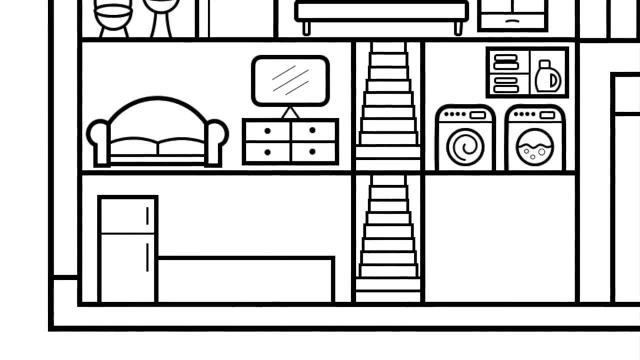 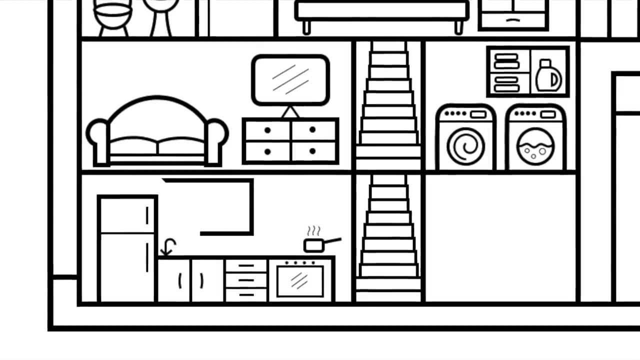 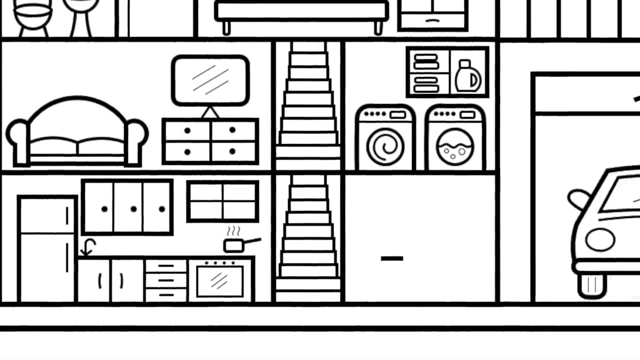 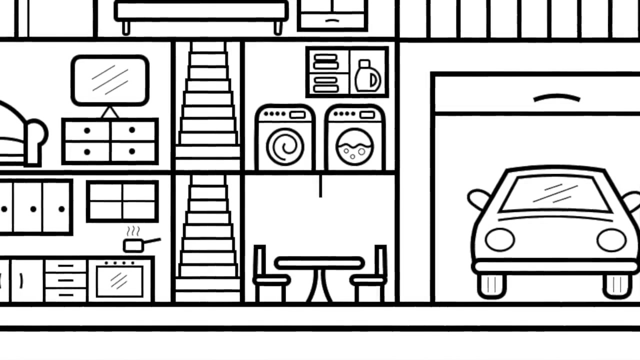 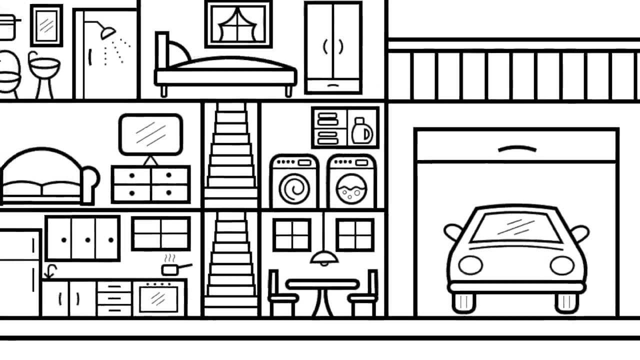 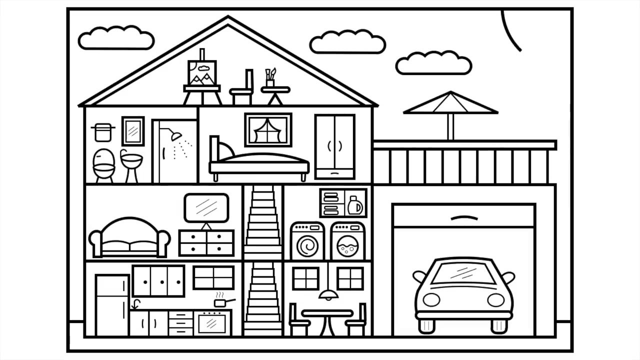 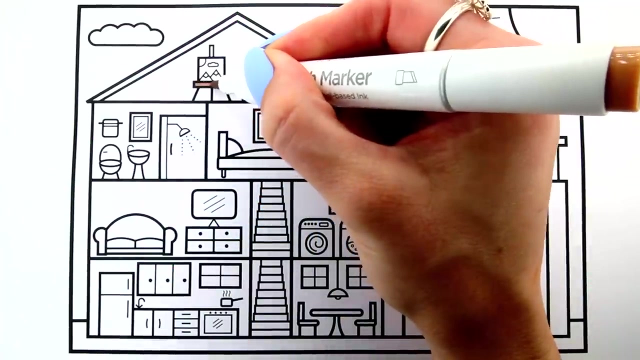 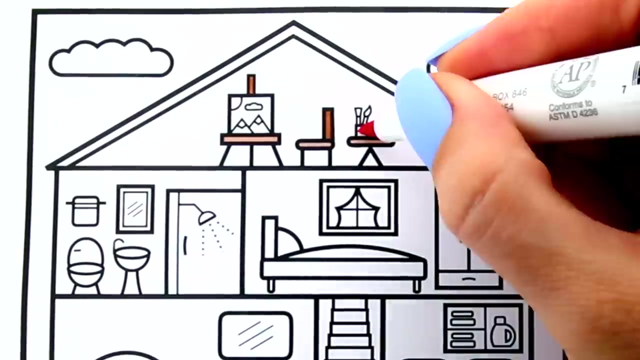 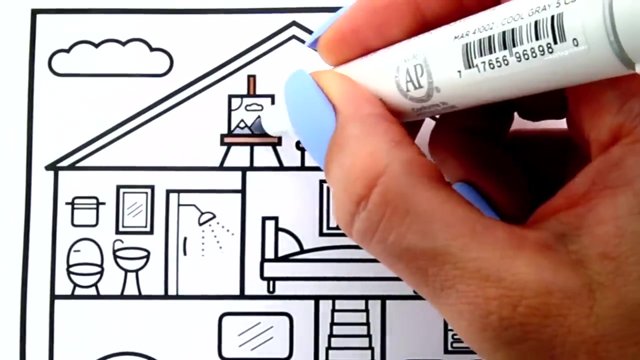 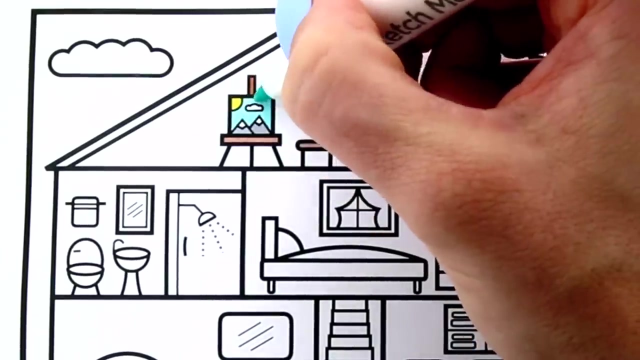 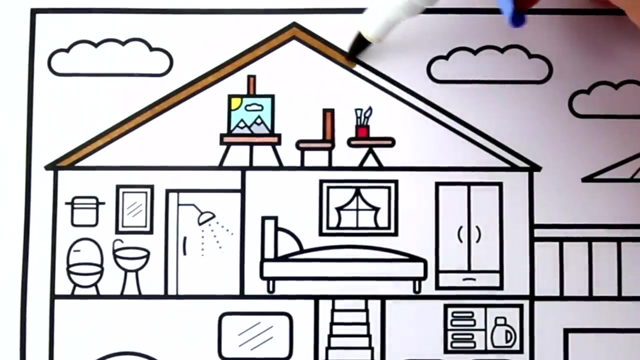 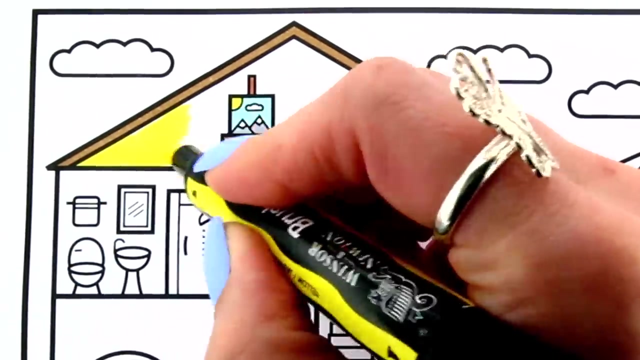 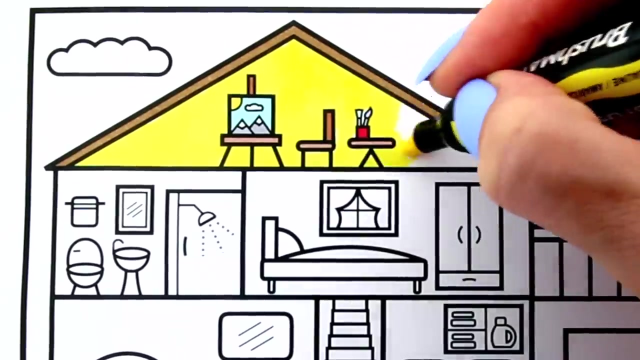 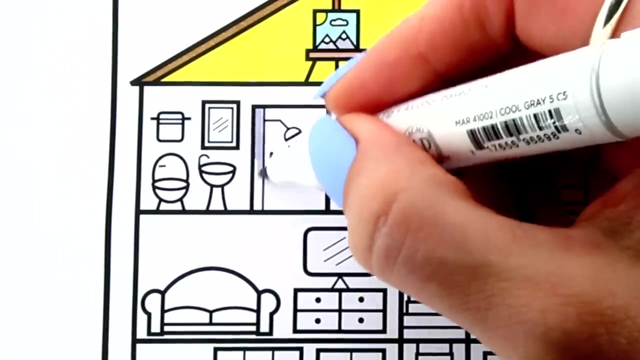 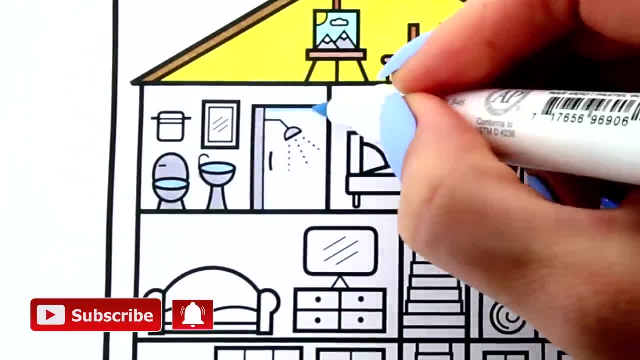 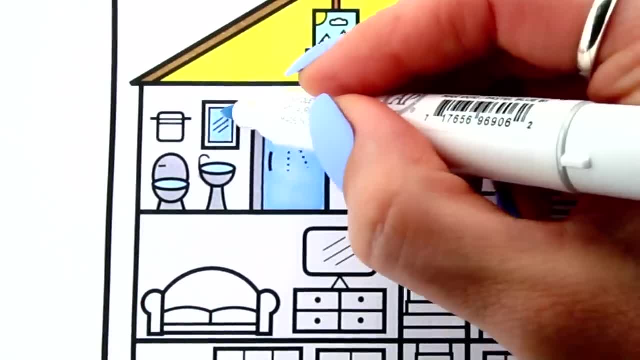 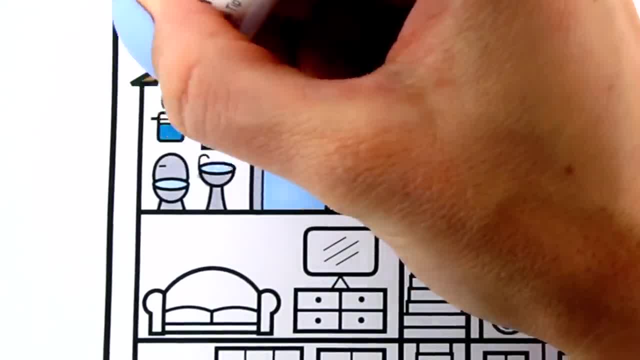 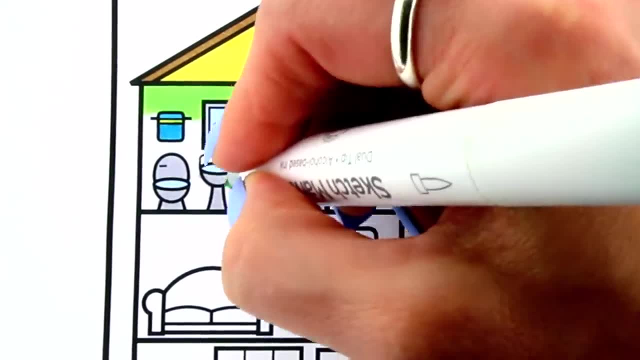 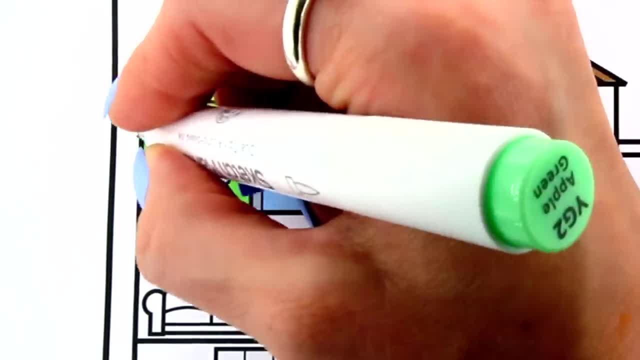 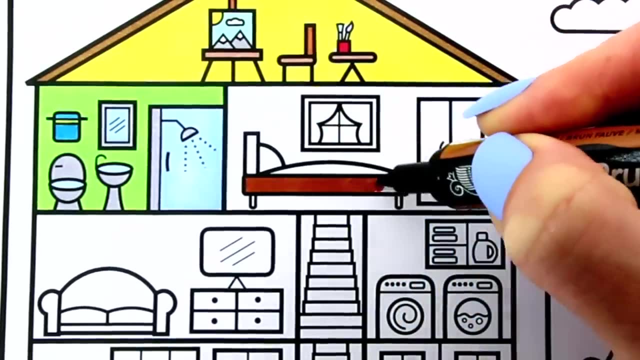 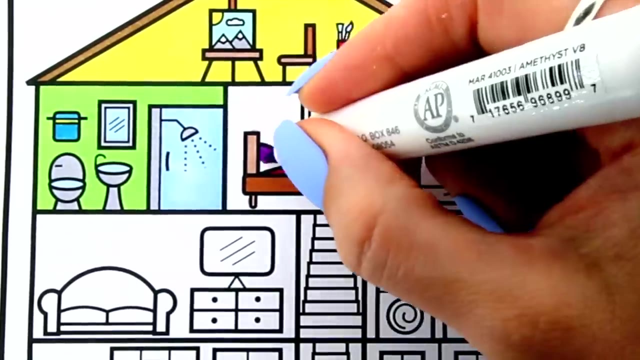 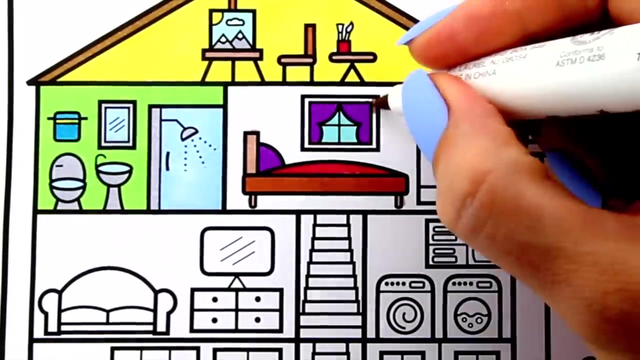 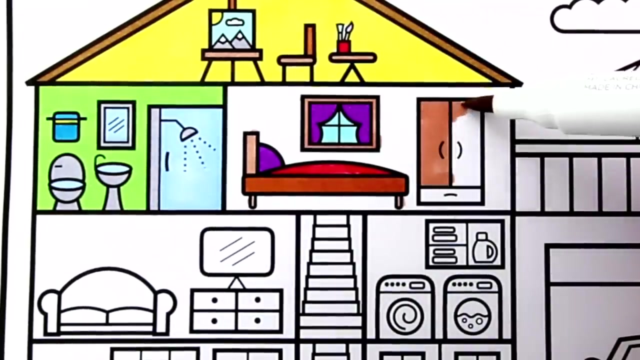 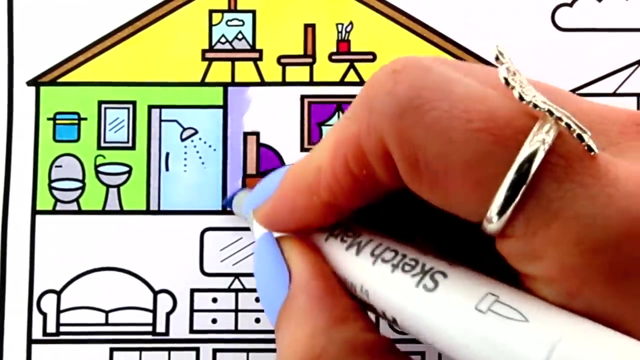 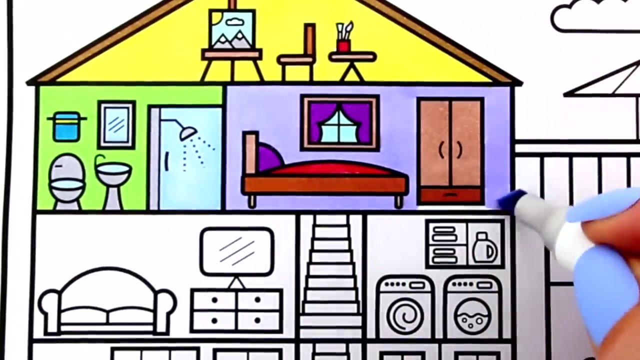 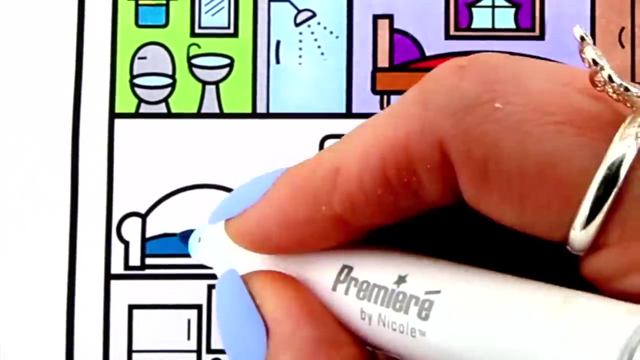 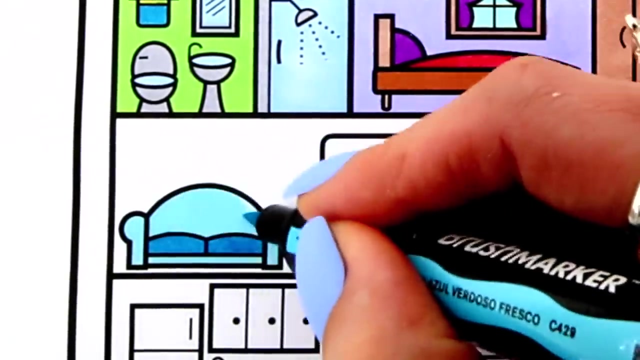 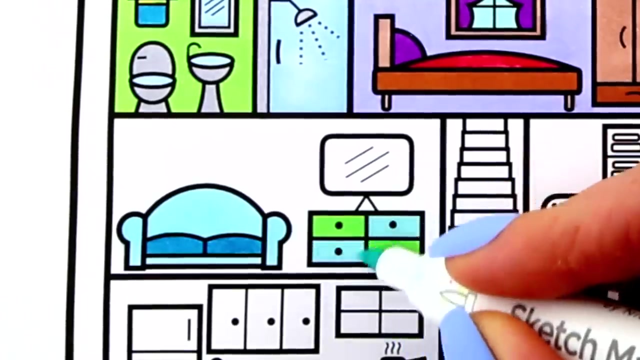 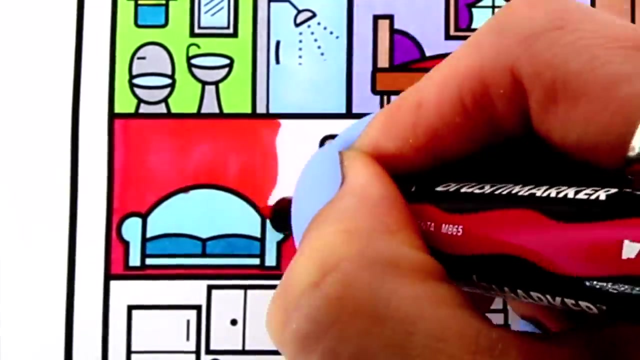 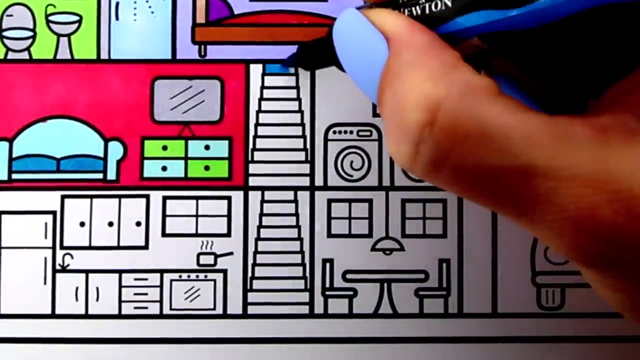 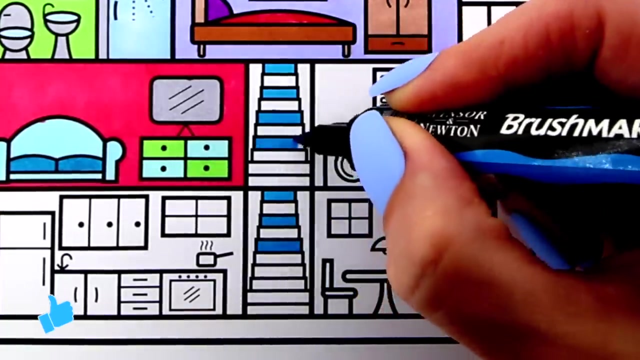 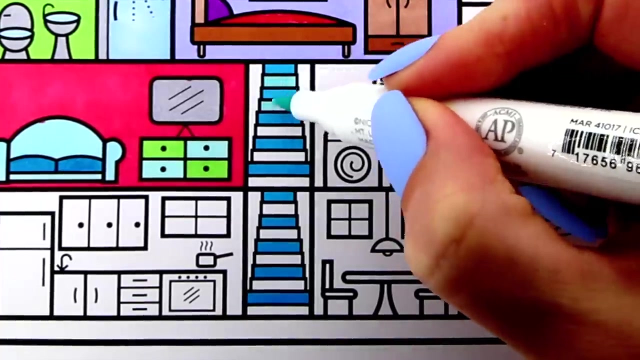 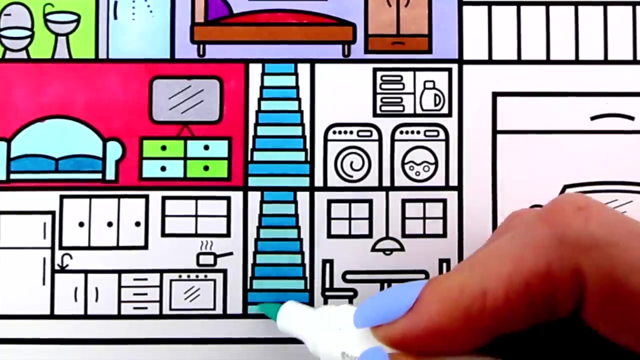 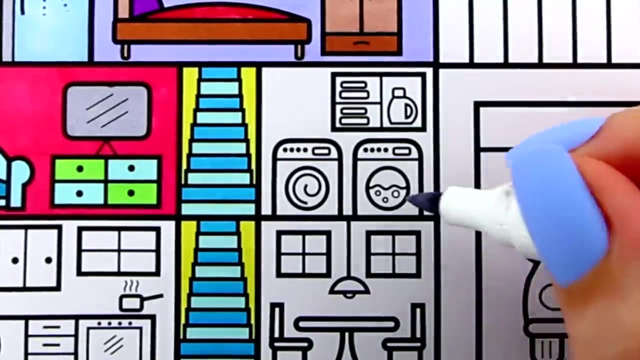 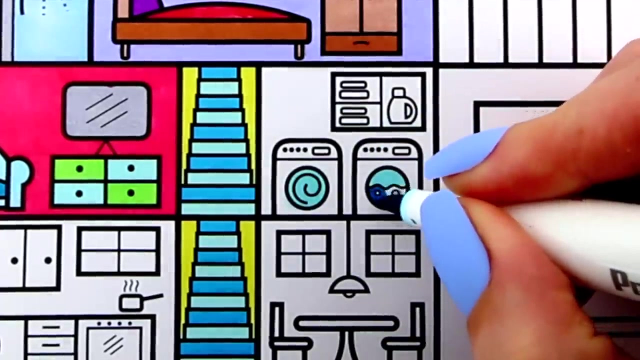 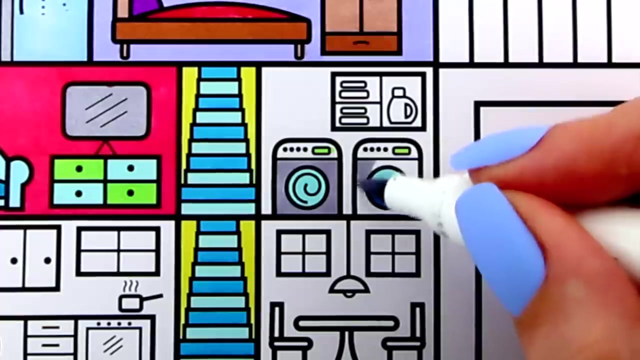 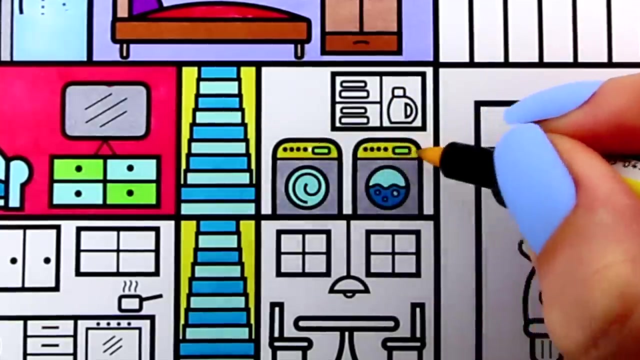 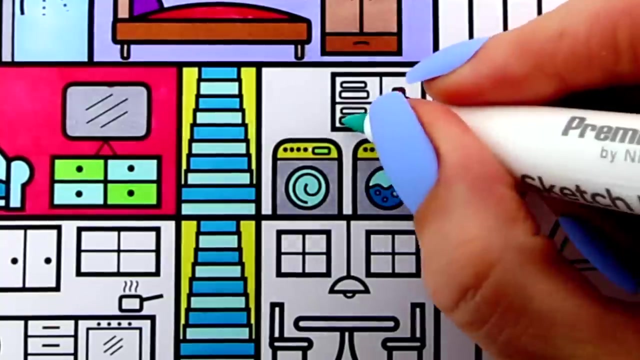 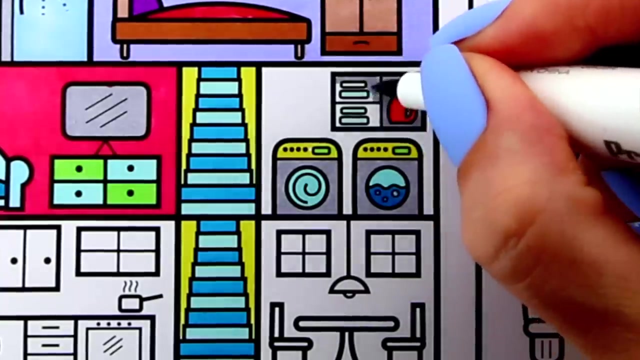 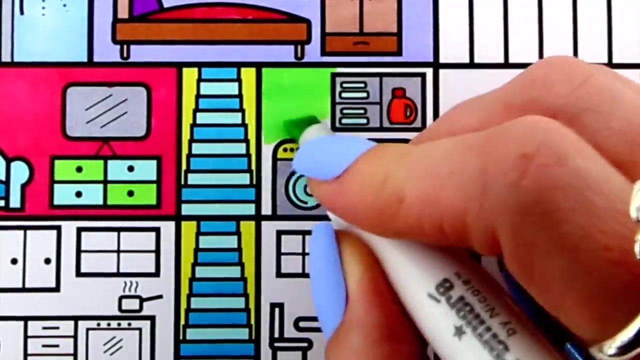 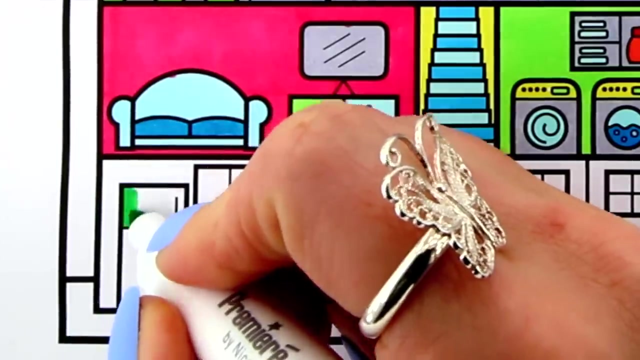 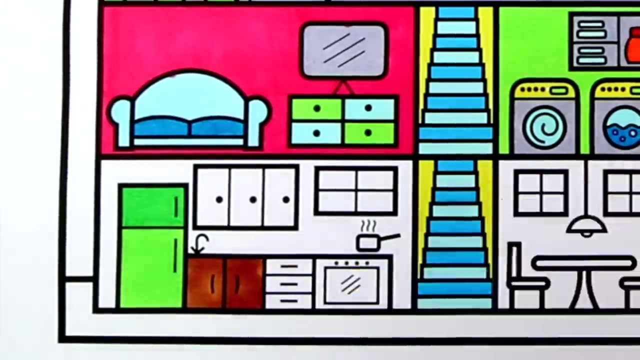 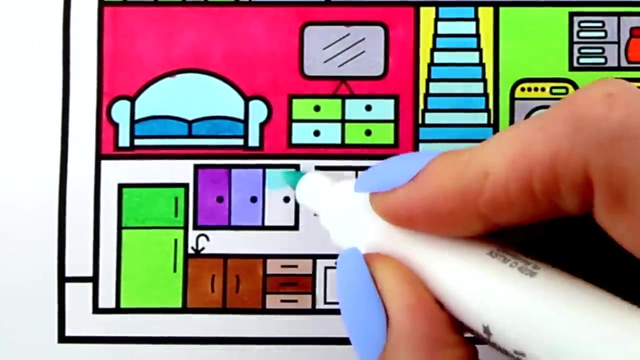 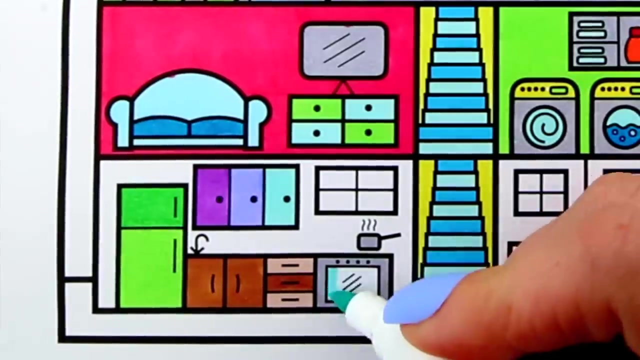 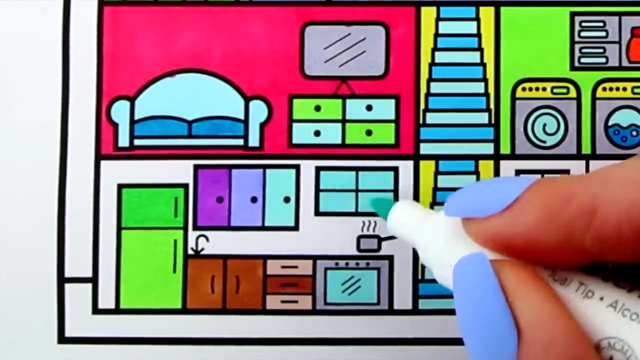 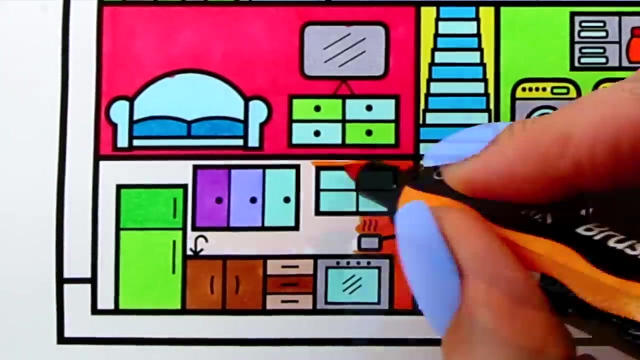 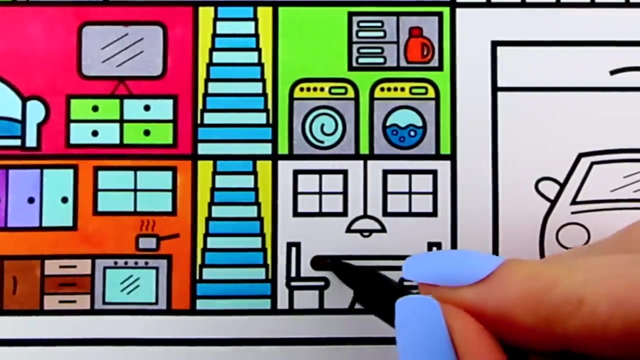 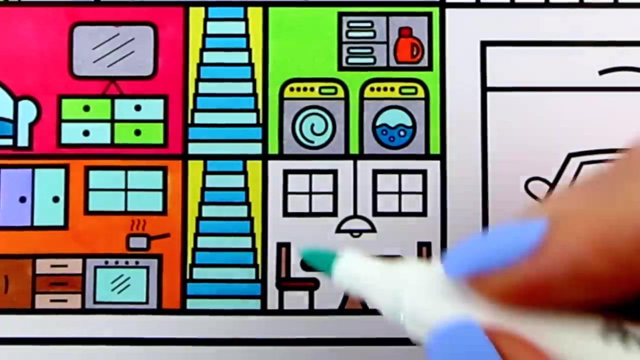 Let's get started. Thank you. Thank you, Hi everybody. If you like this video, please give it a thumbs up. Thank you. If you like this video, please give it a thumbs up. Thank you. If you like this video, please give it a thumbs up. 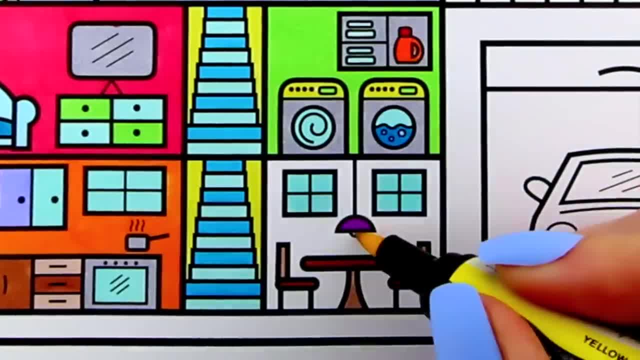 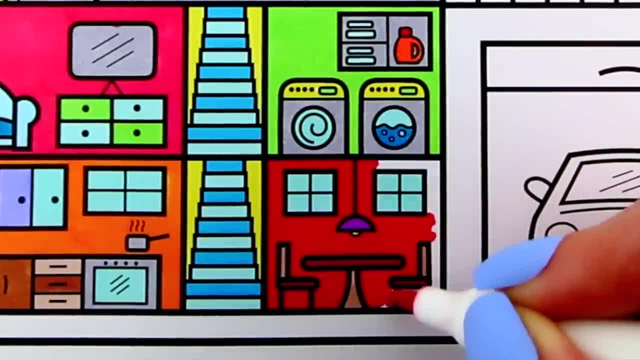 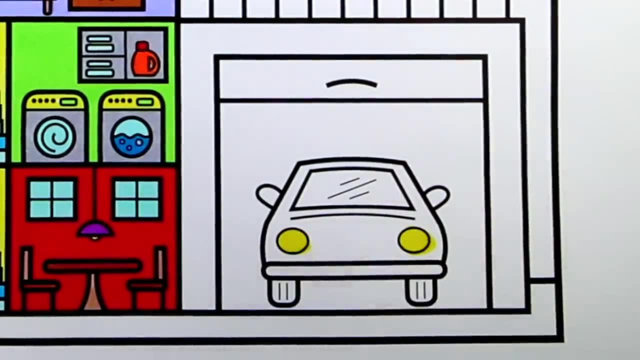 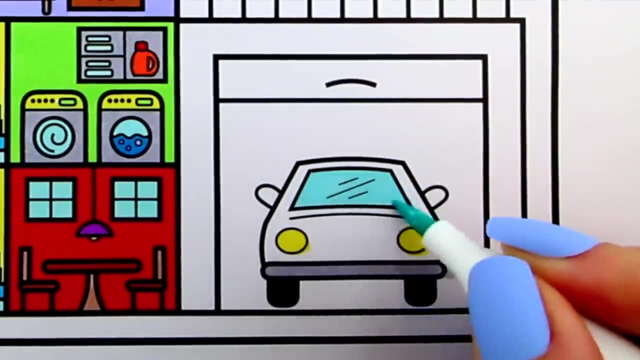 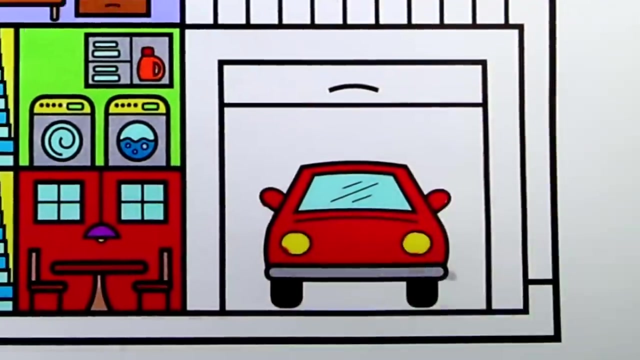 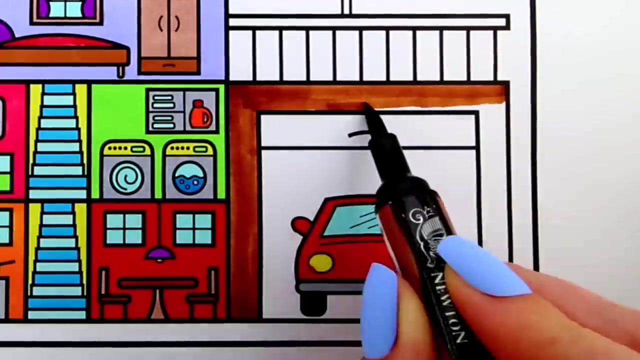 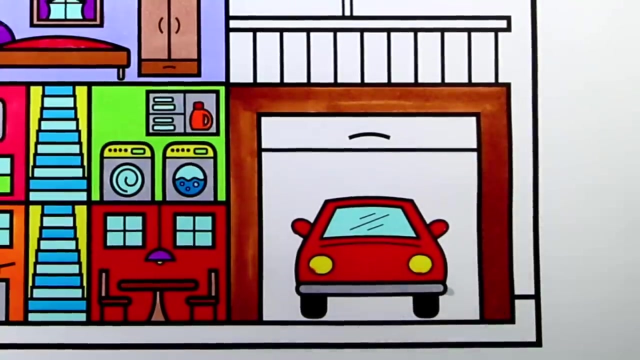 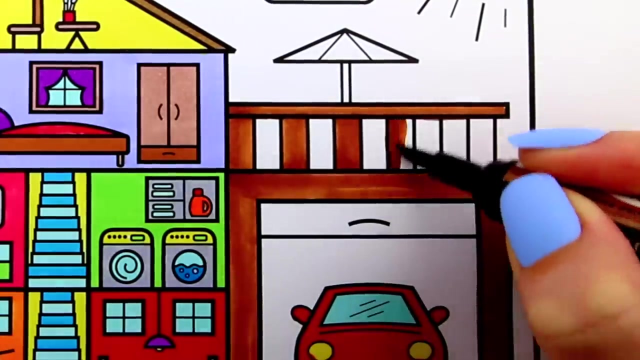 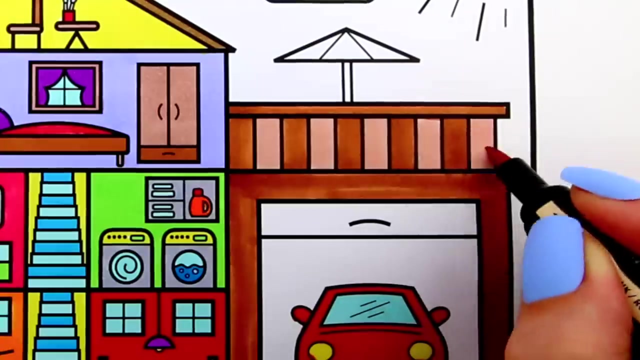 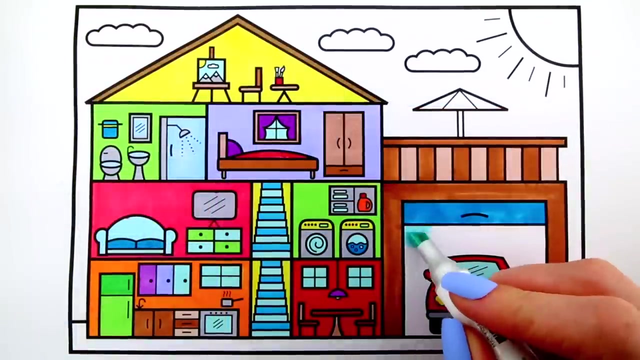 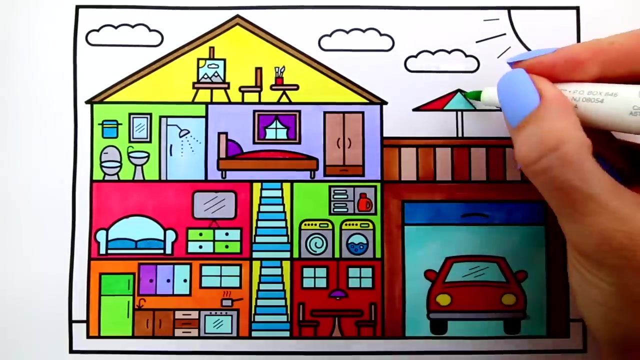 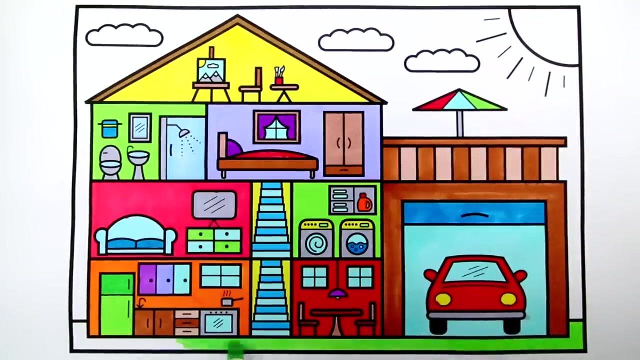 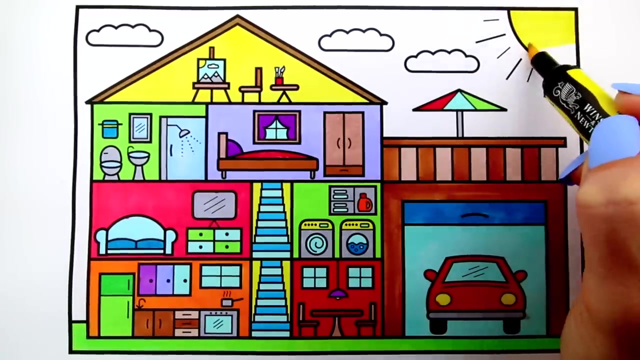 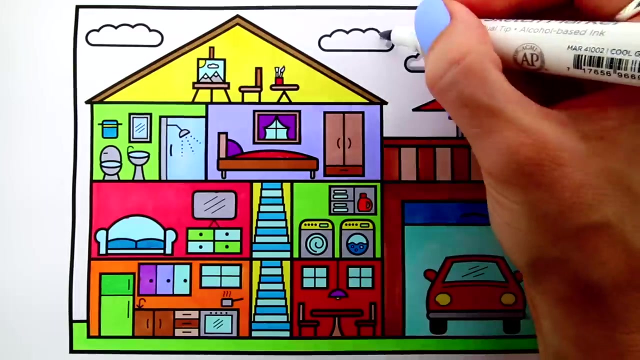 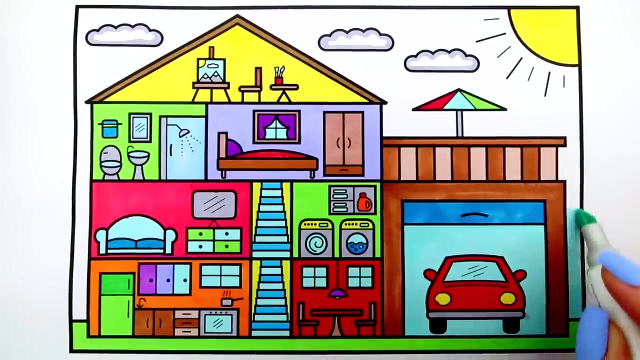 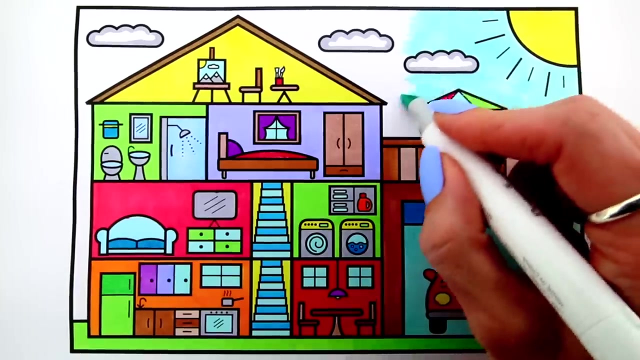 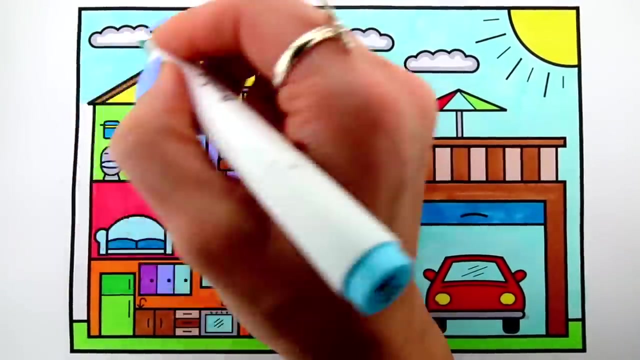 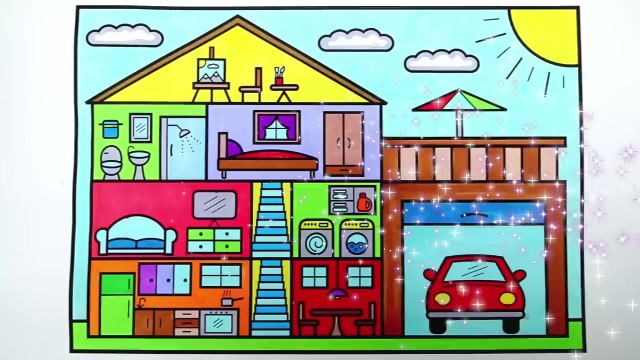 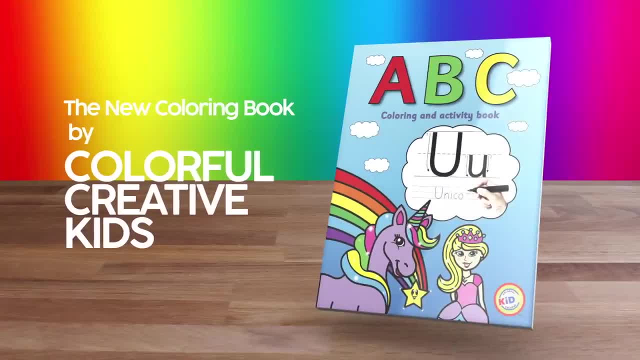 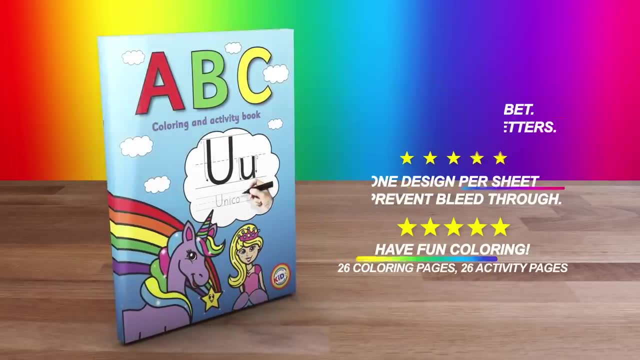 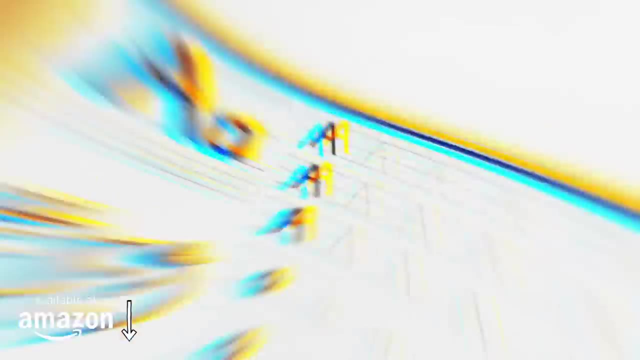 Hey, colorful, creative kids family, If you have been enjoying our coloring pages and original designs, please check out our new coloring books available on Amazon. They include some of our most popular pages and now you can color along with us at home. Thank you. 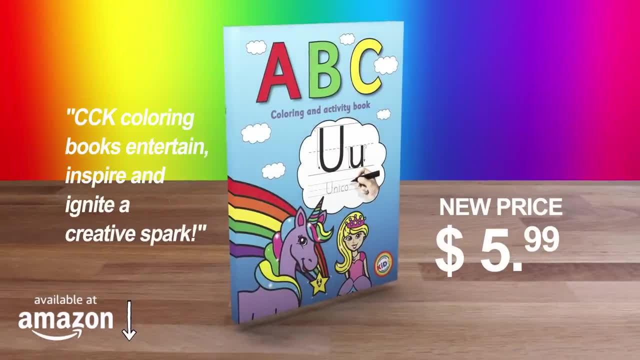 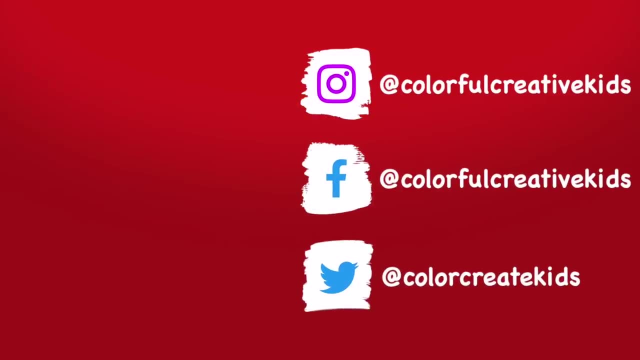 just click on the Amazon link in the description section down below. also, please share your masterpieces. just take a picture of your completed and colored cck page and have your parents share with us on social media. thank you so. 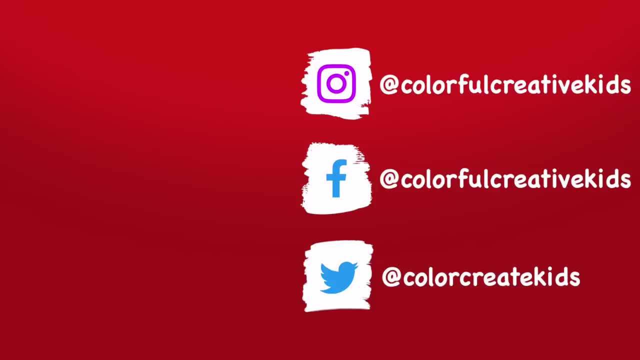 much for watching and we'll see you in our next video.